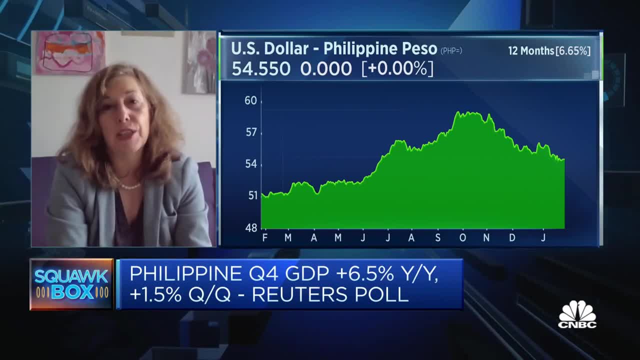 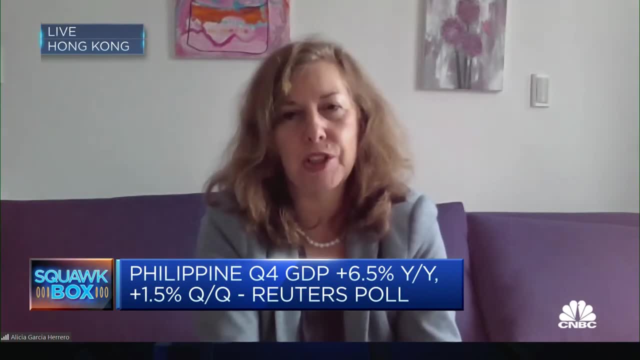 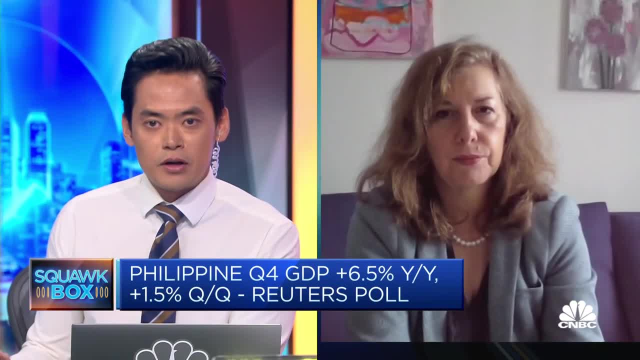 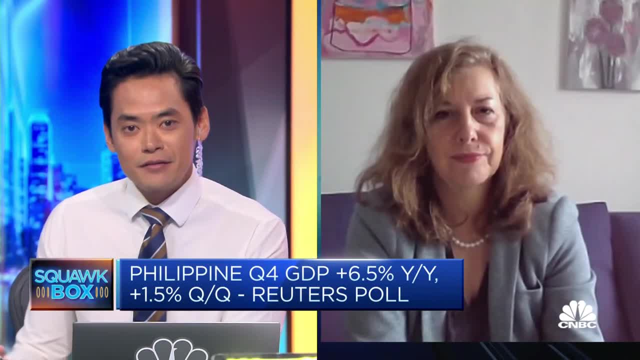 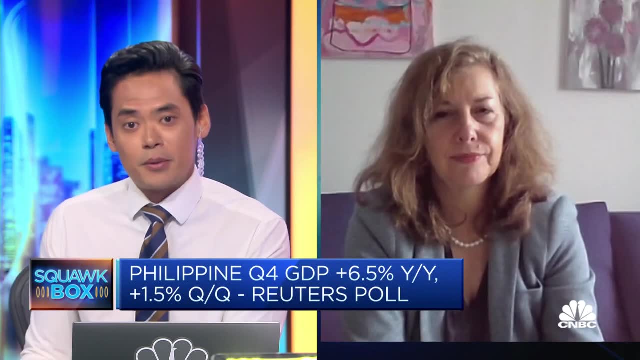 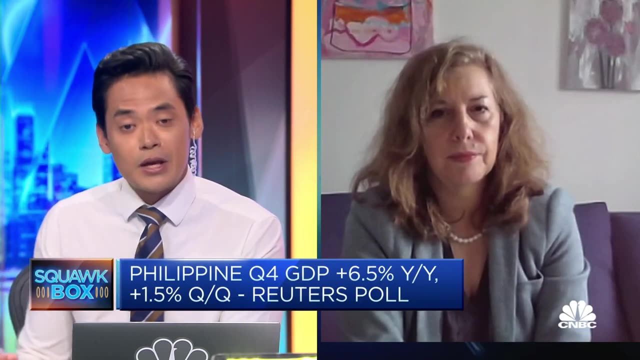 growth, but if inflation continues to stay quite elevated for the Philippines, how might this actually dent or perhaps complicate the efforts by the bank or other economic officials in terms of controlling inflation and while not trying to endanger consumer sentiment, which is very important in terms of that economy in that eastern part of southeast Asia? 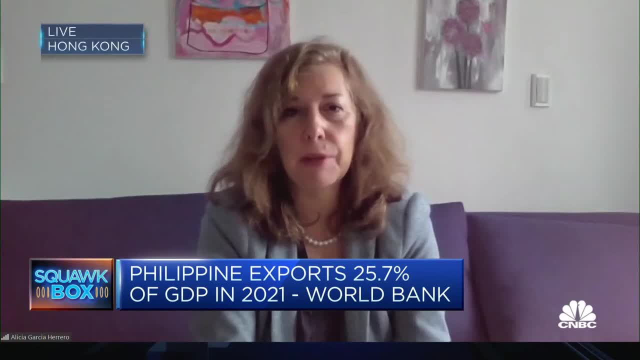 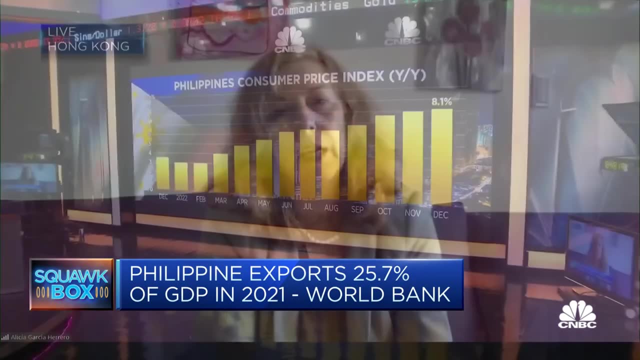 no, you're absolutely right. that's the key risk for the Philippines, I mean for many. it's, like you know, basically US growth, you name it. for the Philippines, it is really inflation. a lot of the inflation, as we surely know, is about food inflation and energy inflation. the Philippines is 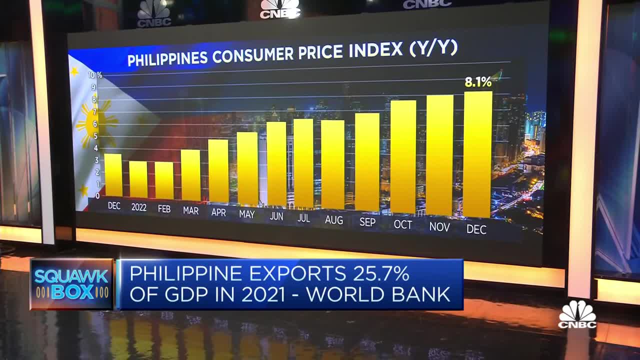 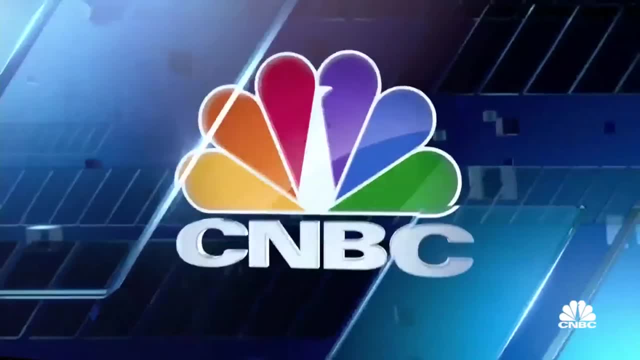 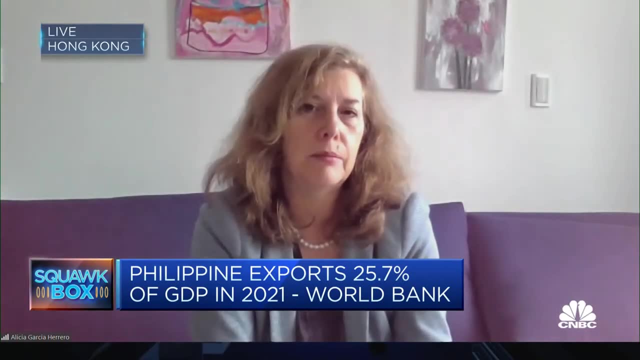 absolutely dependent on on on overseas, whether it's actually food, rice, but especially oil, and and that means that if those prices- which is basically the consensus- will not increase further, we just need basically oil to stay stable, not to have inflationary pressure on on oil demand from. 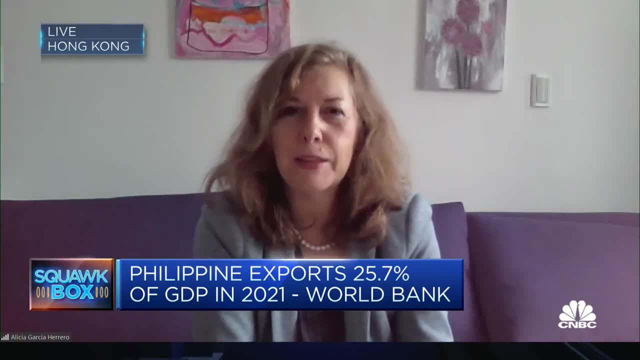 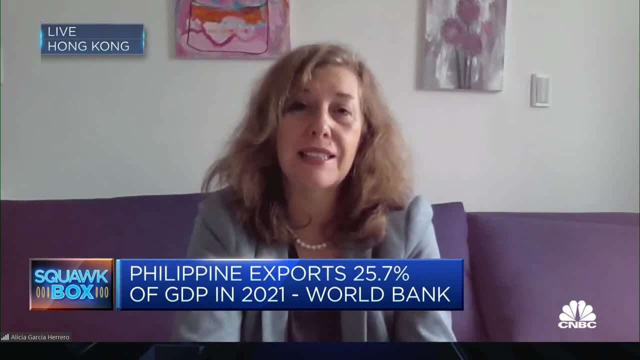 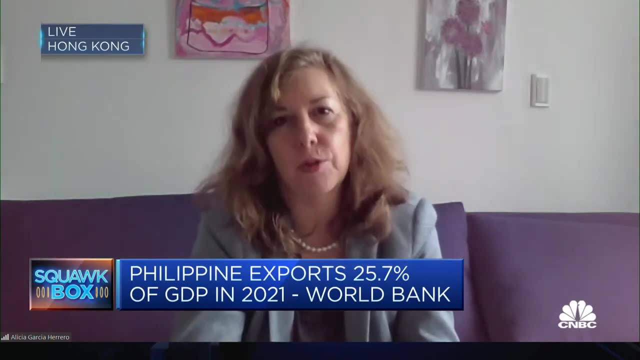 Marcos in Davos and Marcos in Beijing basically trying to secure more oil- Marcos in Davos and Marcos in Beijing basically trying to secure more oil tourism. but it's much more important that China doesn't grow too much, because that too much would mean an additional push on energy prices would deter, as you rightly.